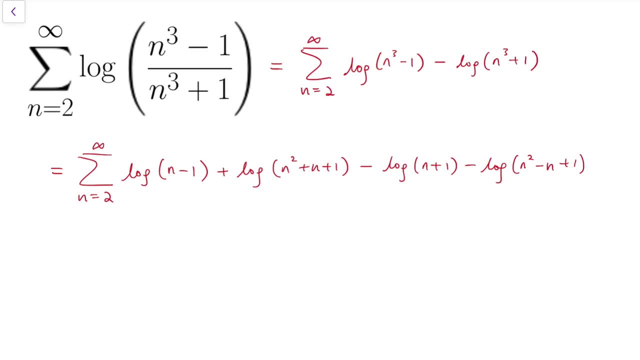 n plus 1.. Simply factorization. Next, I'm going to split it into two summations: One dealing with the log of the linear term, log of n minus 1 minus. log of n plus 1 plus n squared plus n, bigger than log of n square plus n plus 1,. 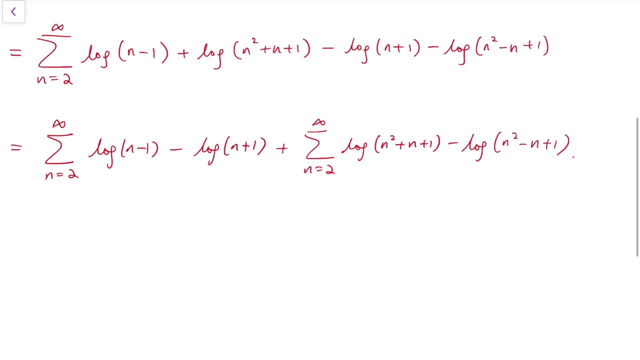 minus the logarithm of n squared more than n squared minus n squared n squared minus n plus 1.. Now we can deal with each of the summations separately. For the first summation, so intuitively, there should be some kind of telescoping sum going on. 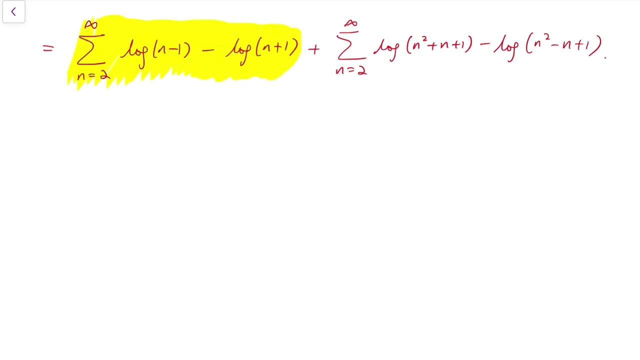 because the first few terms are just drafting log 1 minus log 3, and then we have log 2 minus log 4, log 3 minus log 5, log 4 minus log 6 and so on. Notice that these terms will be cancelled out and you may expect log 5,, 6,, 7,, 8. 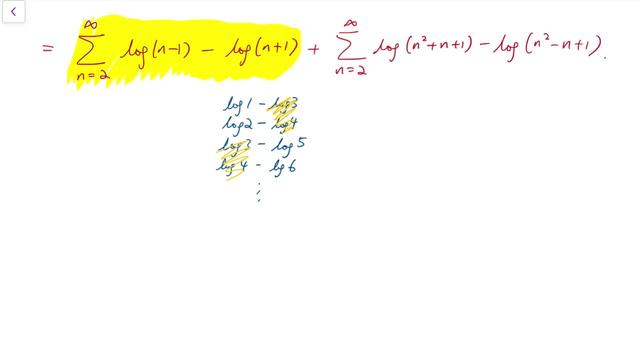 and the terms thereafter should be cancelled out as well. So writing that out rigorously and it will become: the summation of starting from n equals 1 up to infinity of log n, and that's the first logarithm. minus the summation from n equals 3 instead. 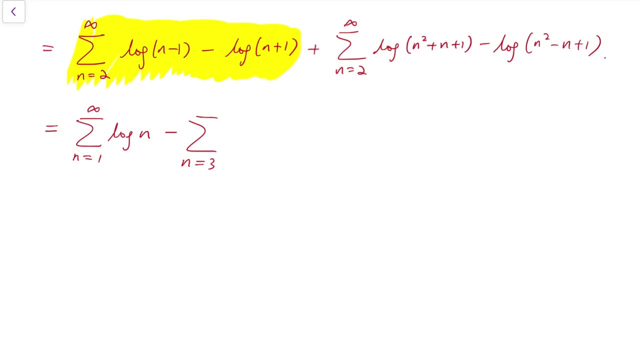 because for the first term it's log of 2 plus 1 and that's actually just 3.. So adding log n again. So for this summation I can subtract and I get just log 1 plus log 2.. So that means we're finished dealing with the summation. 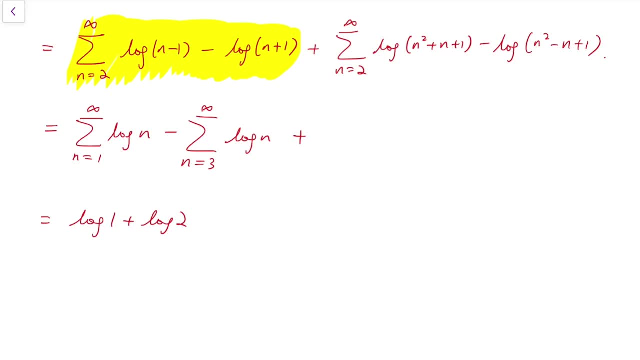 Next we can take a look at the summation afterwards. So, intuitively, we have 2 squared plus 2 plus 1 and that's log 7 minus log 3. Just calculating the values when n equals 2.. Next we have: when n equals 3, we have log 13 minus log 7.. So log 7 cancels out, while for n equals 4. 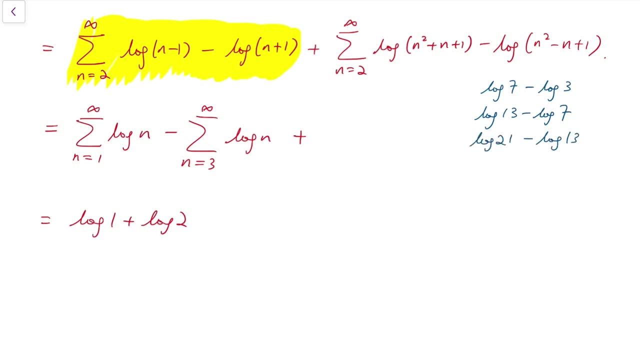 we have log 21 minus log 13.. So again, the log 13 cancels out. So let's see, why would these terms all cancel out? In fact, notice that for a certain value, n, n squared plus n plus 1 takes some numerical value, while for the 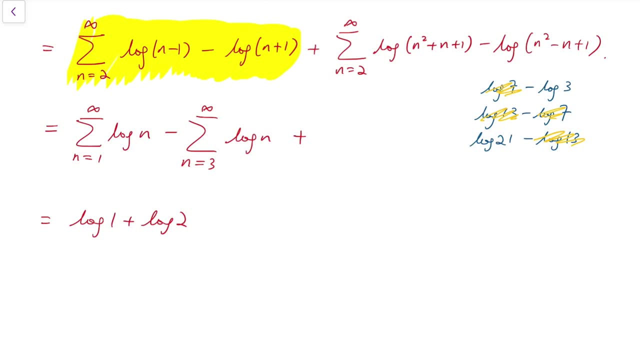 next value of n say next term, say n plus 1. if I put replace n by n plus 1 in this expression, n squared minus n plus 1, let's see n plus 1, all squared minus n plus 1 plus 1 at the end, If we 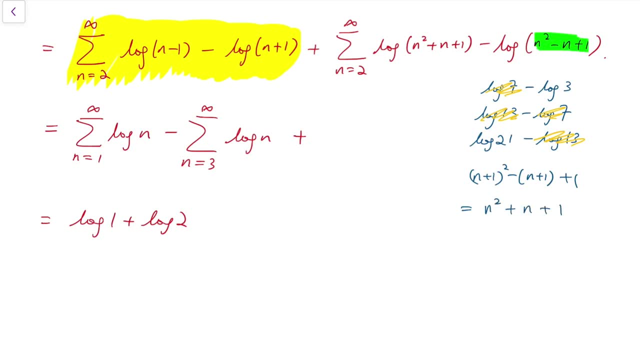 simplify, it's actually exactly n squared plus n plus 1, which is the output of n squared plus n plus 1 in the previous term inside the summation. So that's why we have a telescoping sum happening over here. So to write that out formally, we can do the following Again, adding the summation: 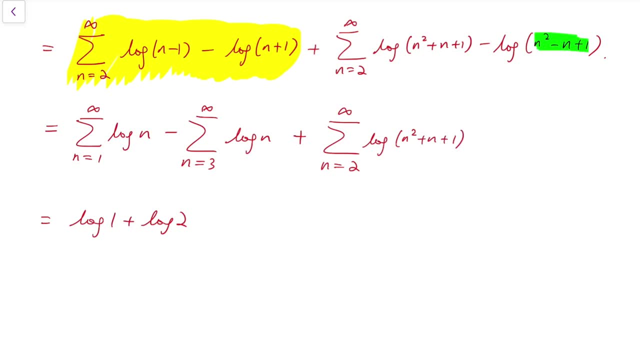 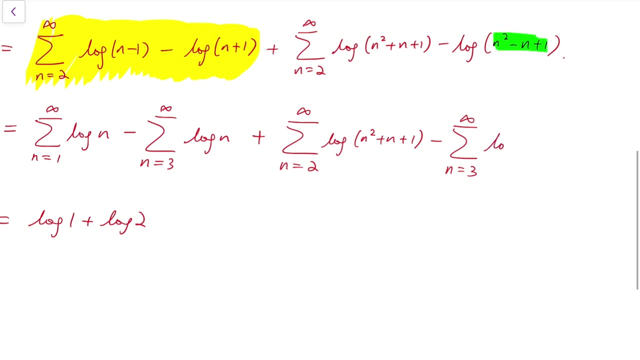 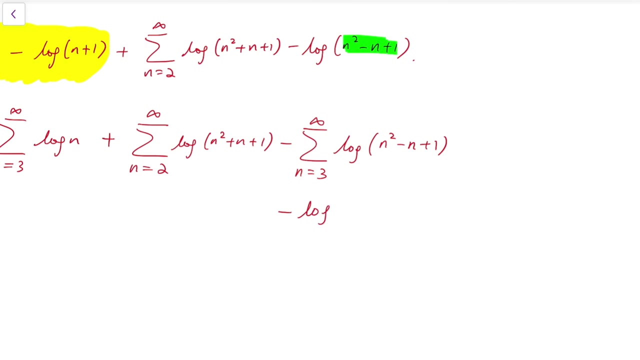 of log of n squared plus n plus 1.. But now I'm going to subtract, when n equals summation, when n equals 3, to infinity of the logarithm of n squared minus n plus 1.. And furthermore, I'm going to subtract another log of 2 squared minus 2 plus 1.. Basically taking out the first term of the.